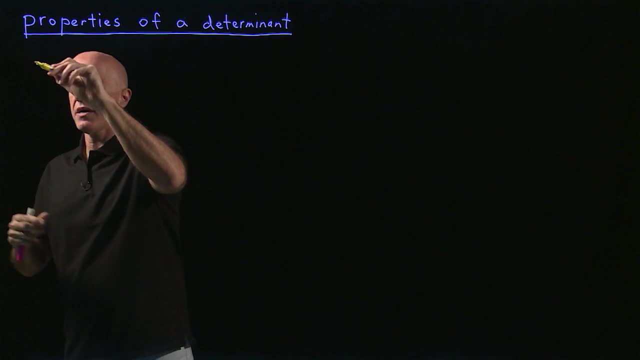 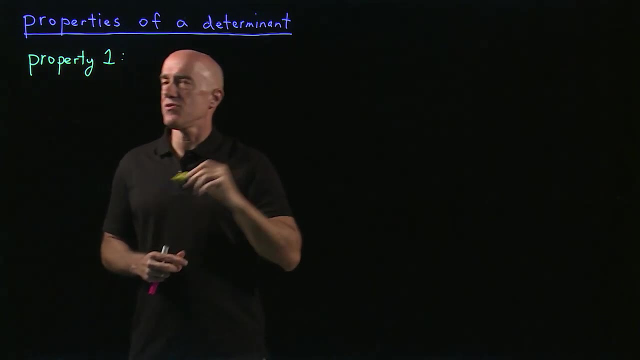 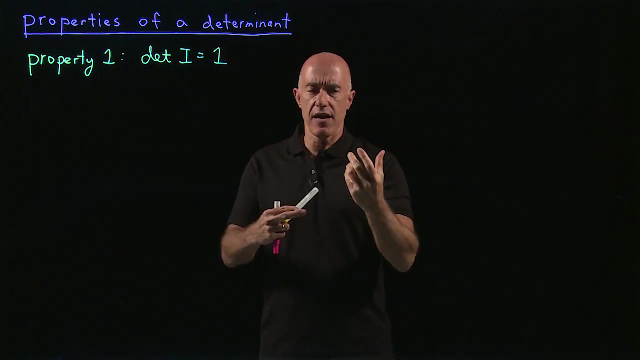 properties. So property one is a normalization property. It's that the determinant of the identity of the determinant is a normalization property. It's that the determinant of the identity matrix equals one. Remember that we introduced the determinant as the number from the matrix. that tells us whether the matrix is invertible or not. If the determinant 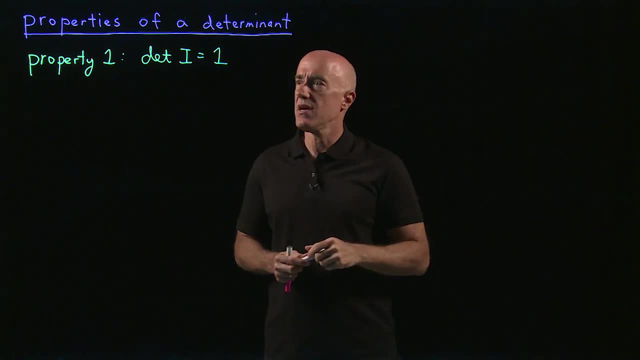 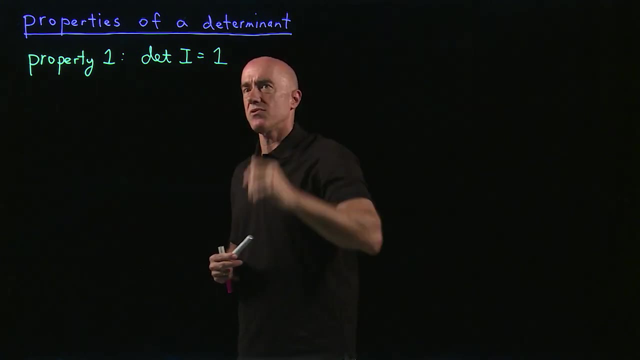 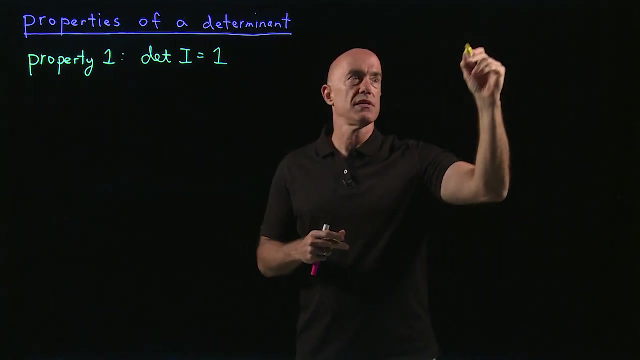 was zero, the matrix did not have an inverse. But you can always, of course, multiply that definition by a constant. So this sets the scale, So this determinant of I equals one. And if I show you The meaning in terms of 2 by 2 matrices, this one is very easy. 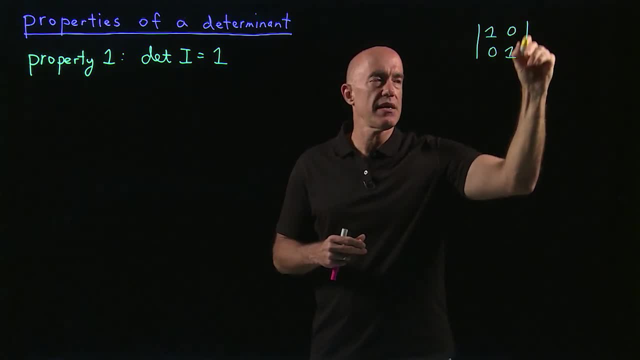 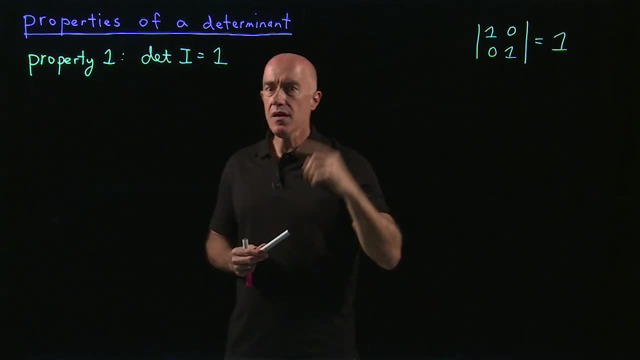 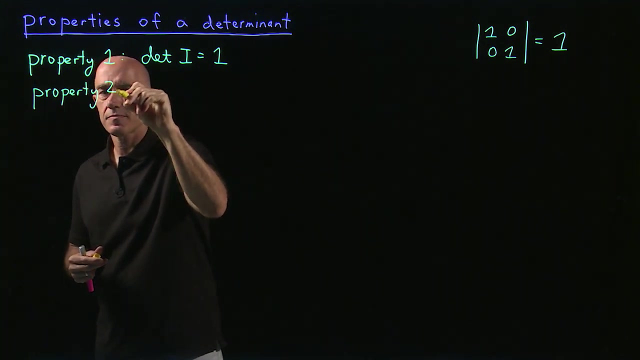 So the determinant of the 2 by 2 identity matrix, we know it's 1 times 1 minus 0 times 0. So that will be 1, right. That's the first property. The second property, property 2, is that the determinant will change sign. 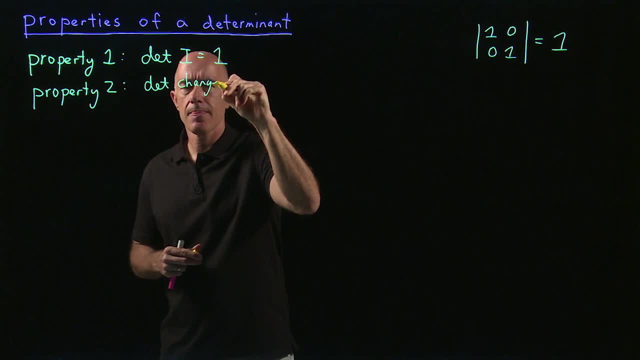 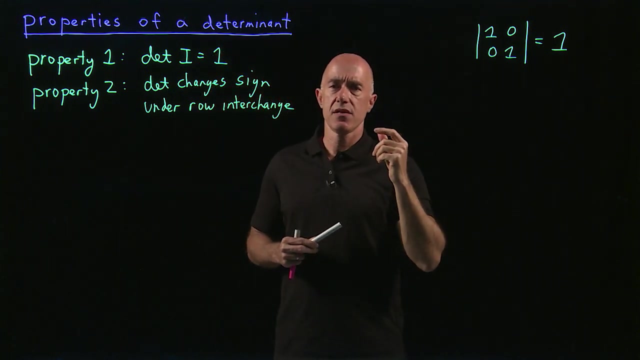 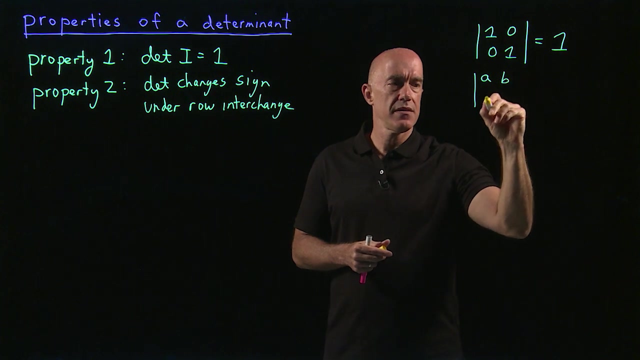 The determinant changes. sign under row interchange. okay, So if you switch two rows in a matrix, the determinant will change. sign Here we can see if we take A, B, C, D and then we switch the rows so we have C. 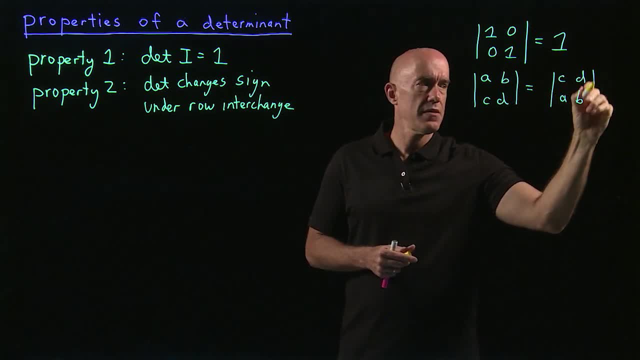 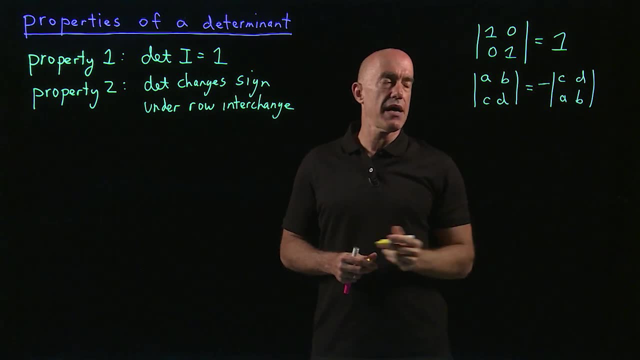 C, D, A B. This is A D minus B C. This is B C minus A D. So this has a minus sign. okay, So the determinant changes sign when you switch two rows. That's a defining property, okay. 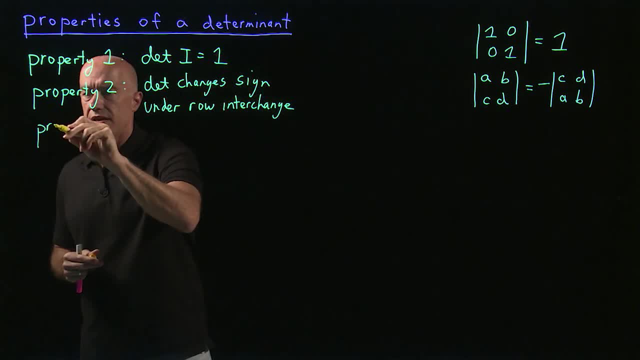 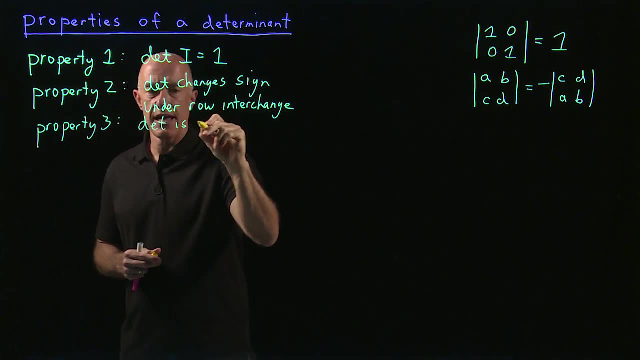 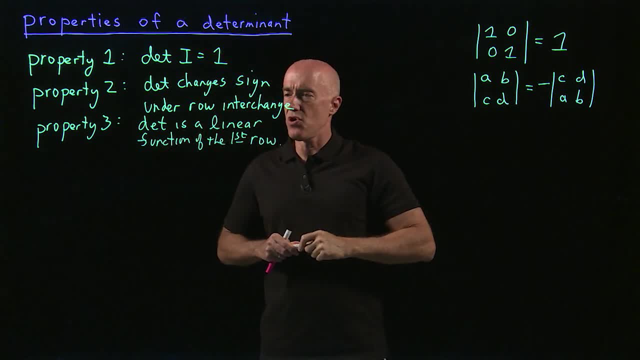 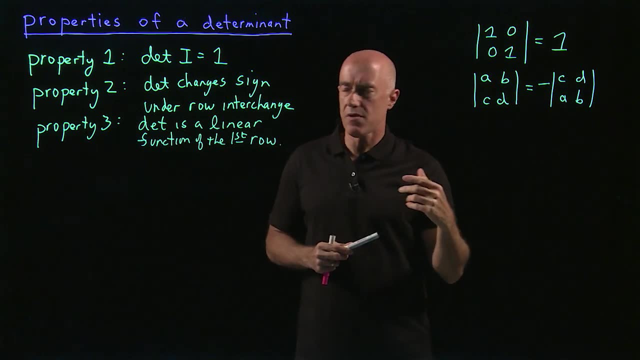 That's a more abstract property that you might not know what I mean by saying the determinant is a linear function of the first row. But I can show you the example with the 2 by 2 matrix. So if you look at linear function actually has two properties. 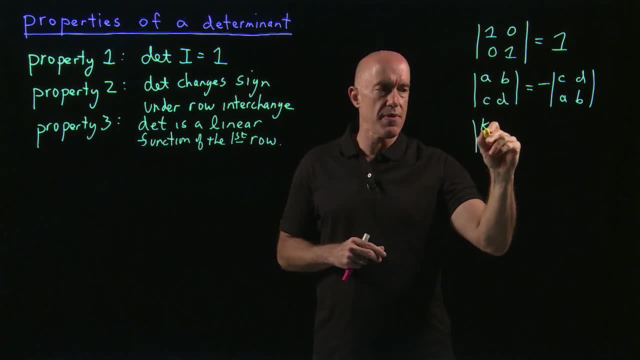 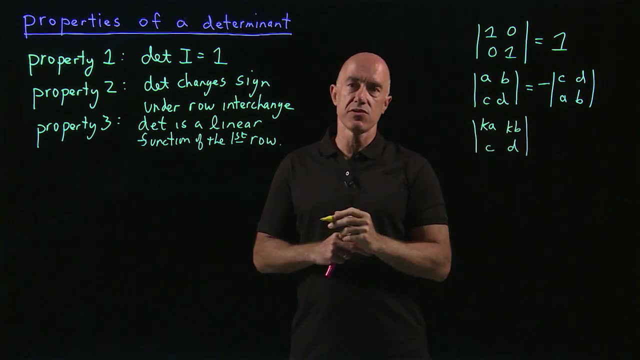 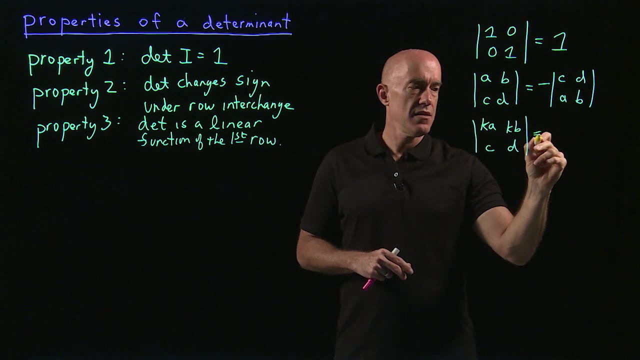 If we look at the linear function, it's a linear function of the first row, the first row, and we multiply it by a constant. so K times A, K times B, C, D, And we ask: what is the determinant of that? We get KAD minus KBC. Both terms have a K in it, so you: 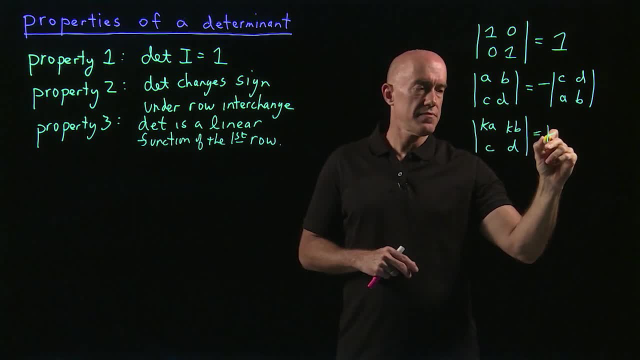 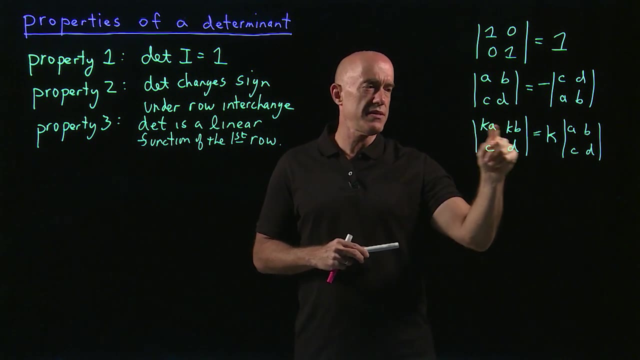 can factor out the K, and then we have A, B, C, D. So saying that the determinant is a linear function of the first row in this instance means that if you multiply the first row only by a constant, keeping the second row unchanged, then you can factor out the. 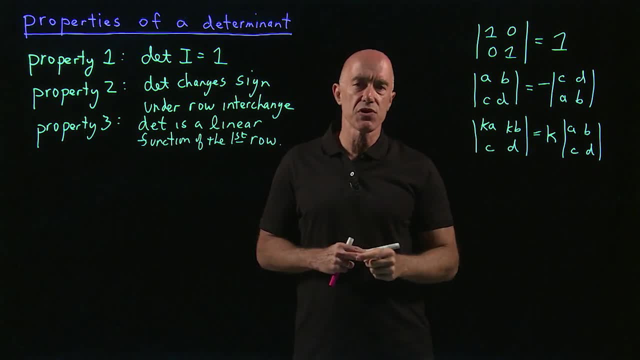 constant. That's different than matrix multiplication, right? Matrix multiplication is: if you multiply a matrix by a scalar, every element in the matrix gets multiplied by the scalar. Here we're restricting it just to one row, keeping all the other rows fixed. Okay, the second. 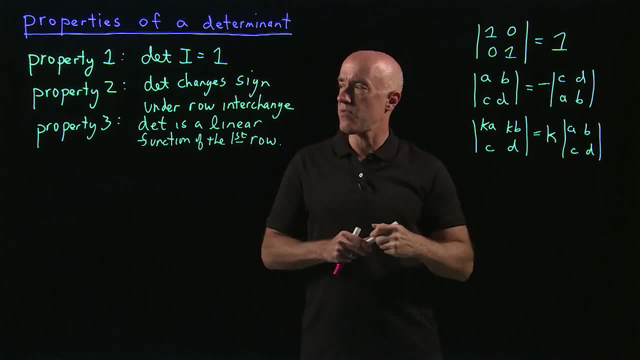 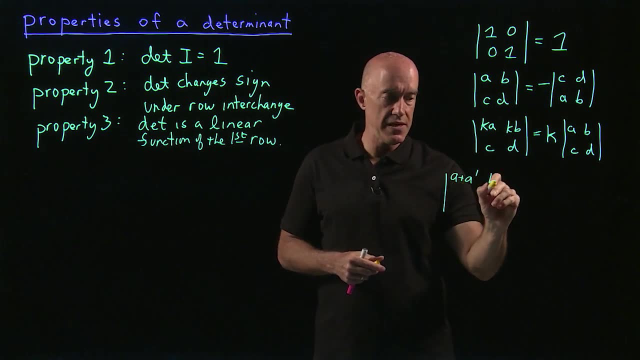 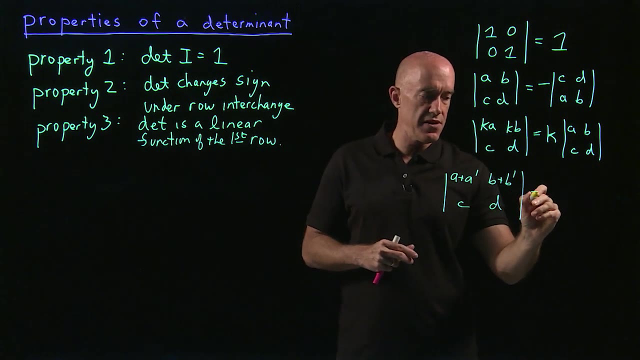 property of a linear function, so these are both property. three is that if we have this matrix A plus A prime B plus A, prime A plus A, prime B plus A prime A plus A prime plus B, prime C, D, then the fact that this is a linear function means we can split this. 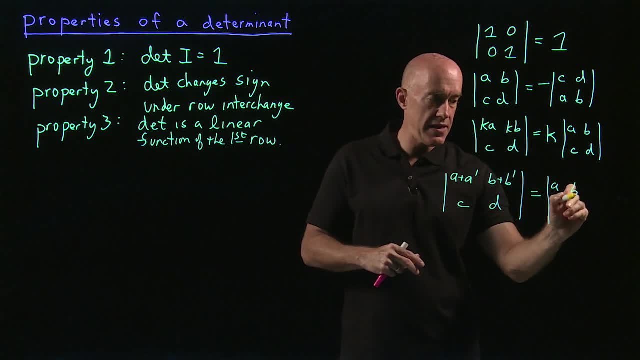 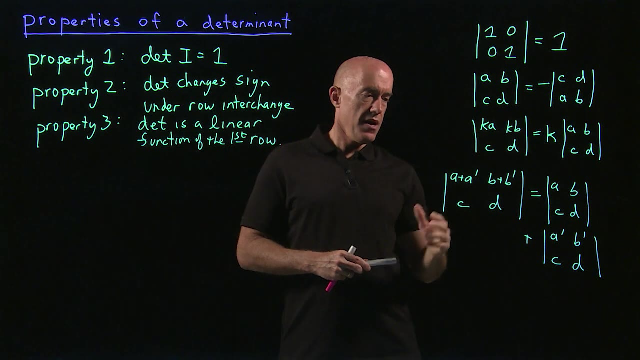 into two determinants: A, B, C D, plus A prime, B, prime C D. So that's the second linear function property. It's a little bit. you can do the algebra to show that it's a linear function. 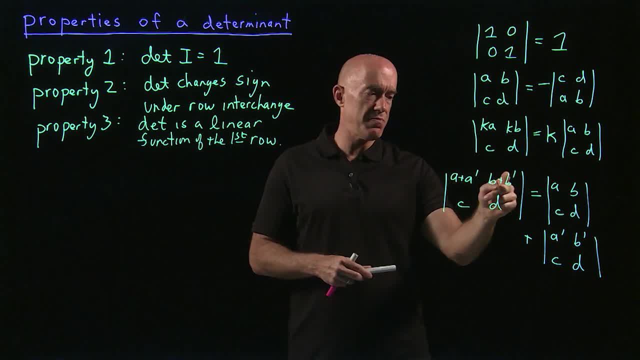 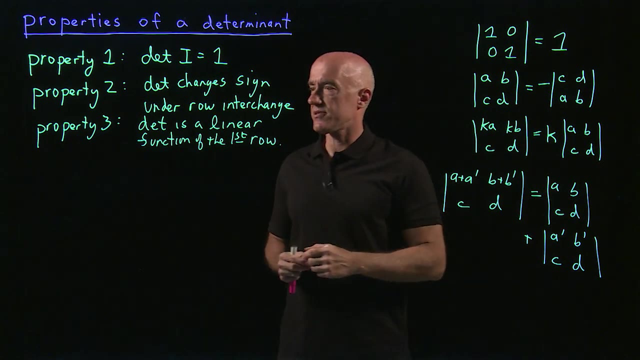 So you can show this right: This is A plus A prime times D minus B plus B prime times C, And then you use the distributive law and then you'll show that you can write that as the sum of two determinants here. Okay, so fine for a two by two matrix. The beauty. 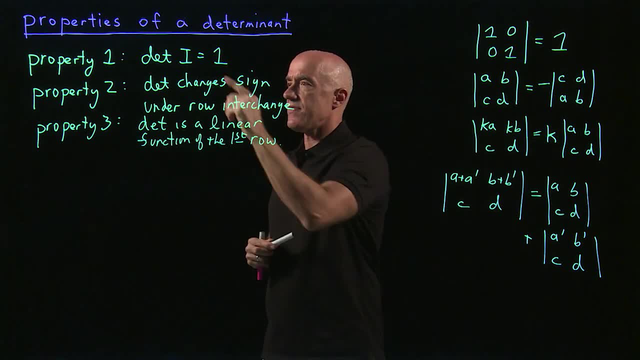 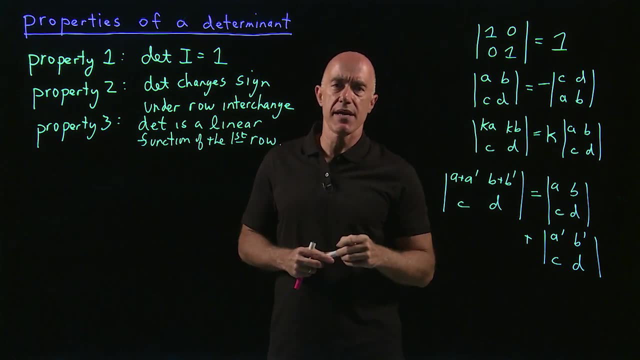 here from a mathematical point of view, is that this is all you need to define the determinant function. Okay, This is a function that maps an n by n matrix to a scalar, to a number. With these definitions you can prove the Laplace expansion, you can prove the Leibniz formula for n by n matrices. 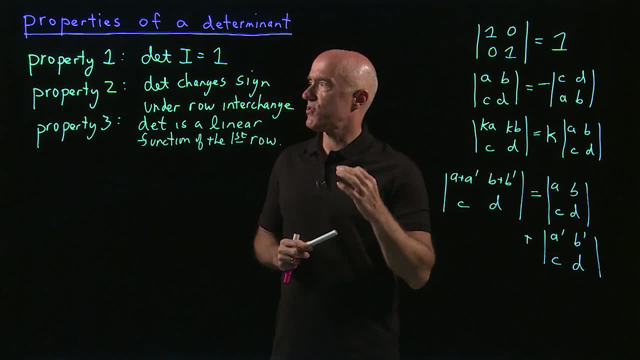 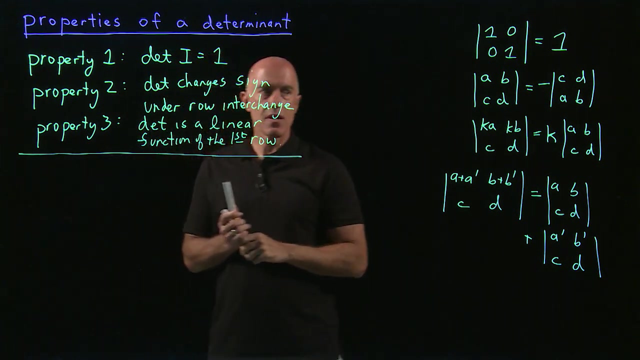 Okay, We won't do that here, but I want to show you that. what are the other properties that these three properties can lead to? Okay, So you can use these original three properties to prove all of these other properties. Let's write down some of these properties. Property three says the determinant is a linear function. 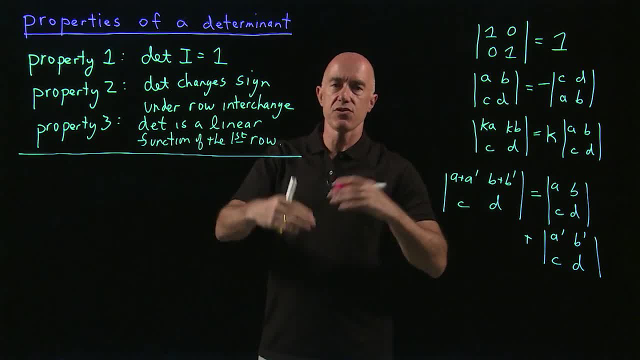 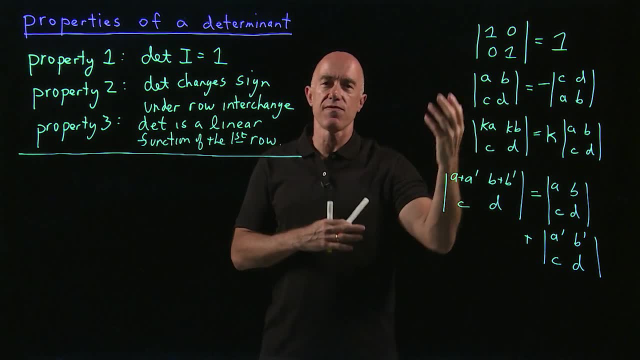 of the first row. but property two says you can interchange rows and change the sign. So if you interchange rows, so let's say you make the second row the first row and then you use that The first row is linear, The second row is a linear function, and then you change the rows back again. then you can. 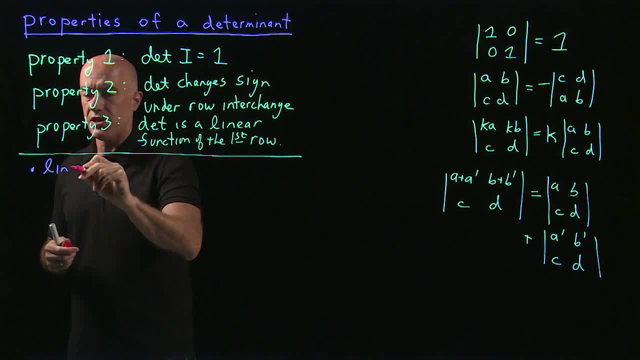 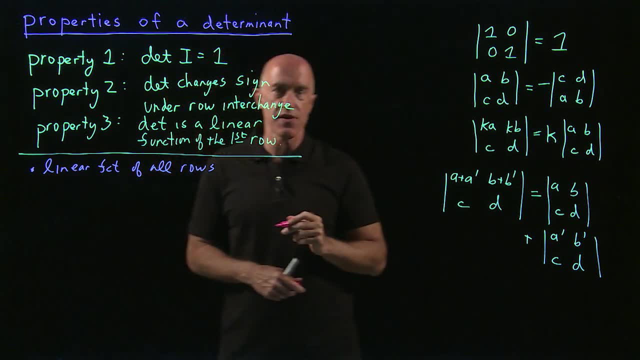 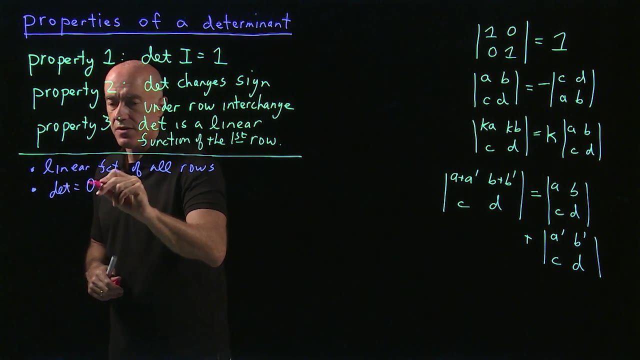 show that the determinant is a linear function of all rows, right, Not just the first row. There's nothing special about the first row. You can prove that the determinant equals zero if you have two rows that are equal, if you have equal rows. 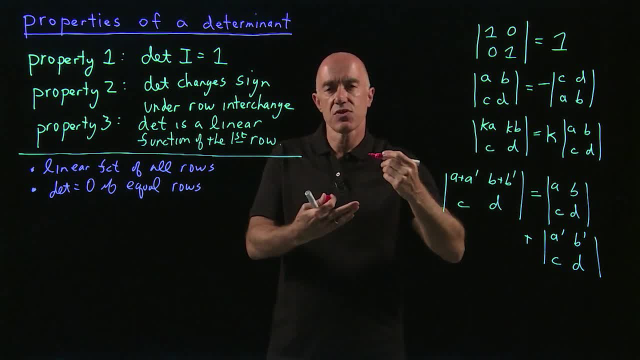 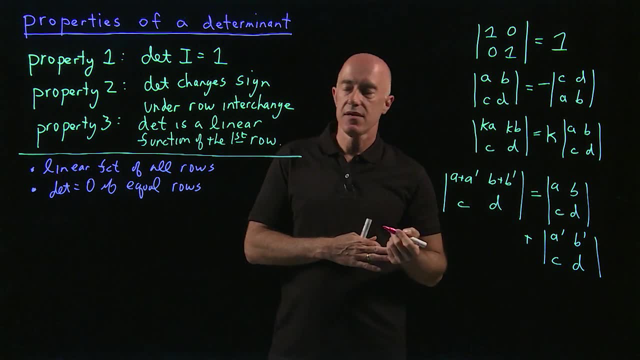 So if two rows are identical, You can switch them. You change the sign of the determinant, but the determinant is the same. So then the determinant has to be zero, right? If x is equal to minus x, then x has to be zero. 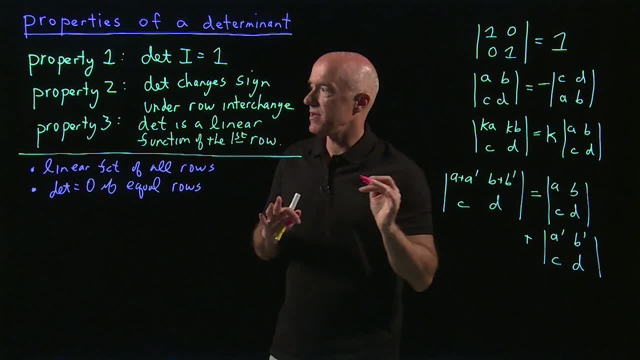 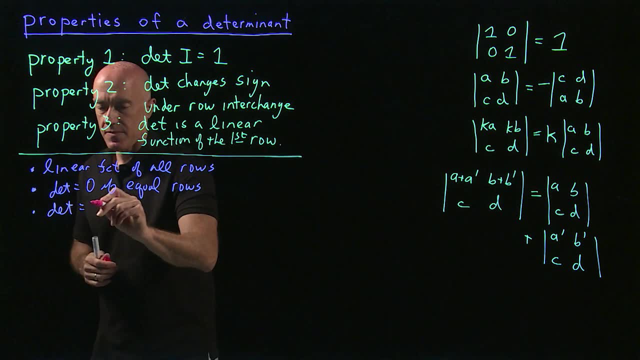 So that's how you prove from these properties. So let me just continue by writing down the properties. The determinant equals zero. If you have two rows, you can change the sign of the determinant, but the determinant is the same If you have a row of zeros. OK, 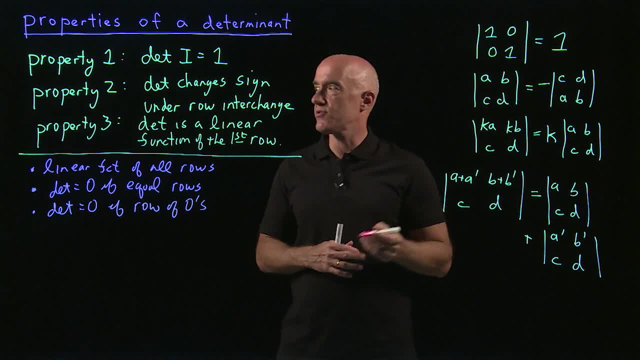 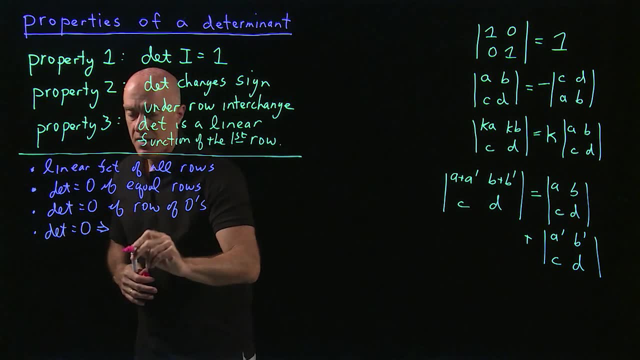 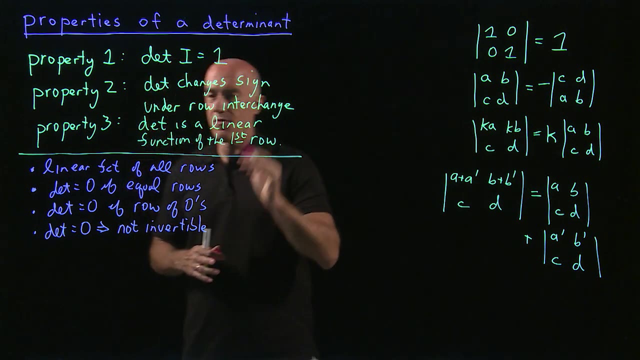 So if one of the rows of the matrix is all zeros, then the determinant is zero. Determinant equals zero, implies not invertible. OK, so that's a very key result, that with these three properties you can prove that if the determinant of an n by n matrix is zero, then that matrix does not have an inverse. 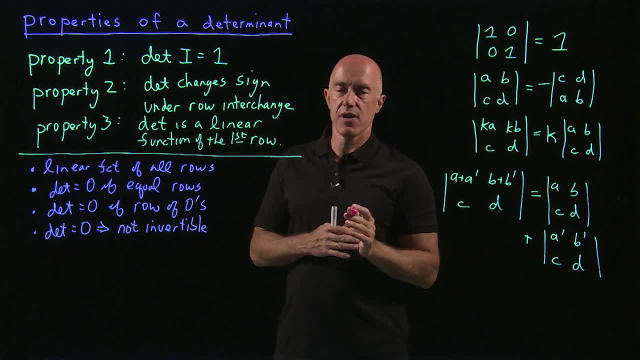 So if you have a row of zeros, OK. So if one of the rows of the matrix is all zeros, then the determinant is zero. OK. so that's a very key result, that with these three properties, you can prove that if the determinant of an n by n matrix is zero, then that matrix does not have an inverse. 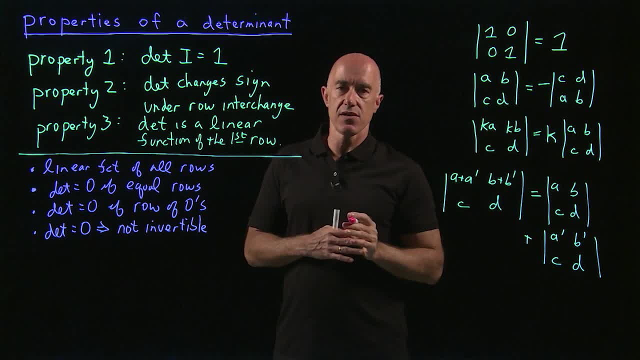 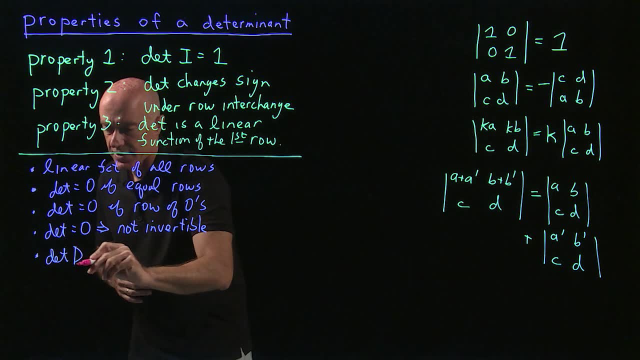 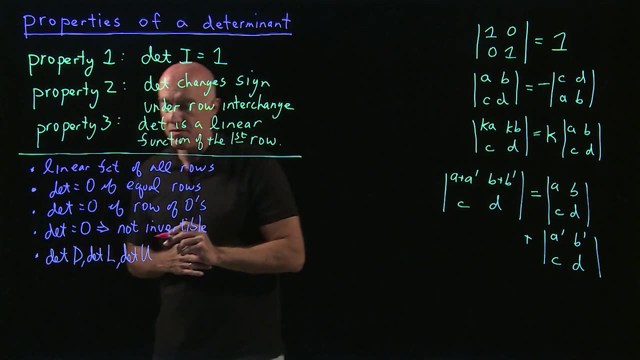 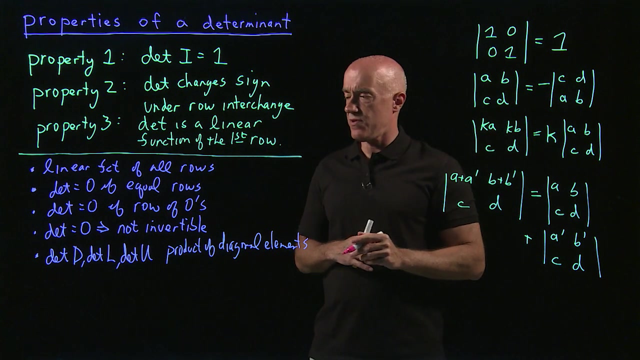 right Ax equals b, does not have a unique solution. The determinant of a diagonal matrix, the determinant of a lower triangular matrix, the determinant of an upper triangular matrix, is just the product of the diagonal elements. OK, So that's from a practical point of view, that's very useful. 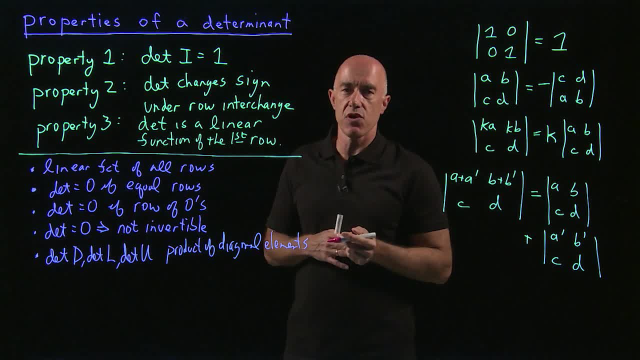 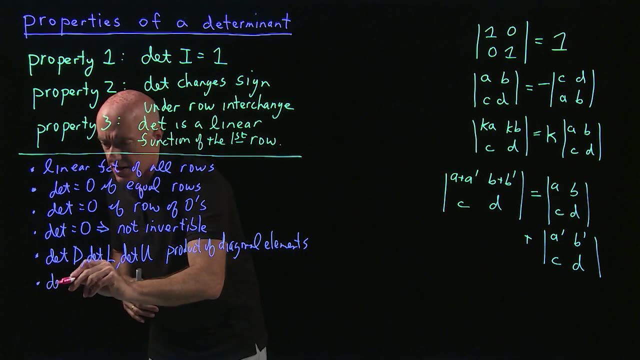 If you can do some operations on a matrix to convert it to an upper triangular matrix, like Gaussian elimination say, then you can just find the determinant from taking the product of the diagonal elements, The determinant of the product of two n by n matrices a times b. 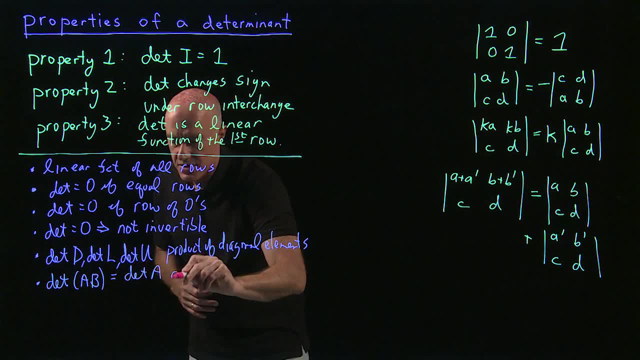 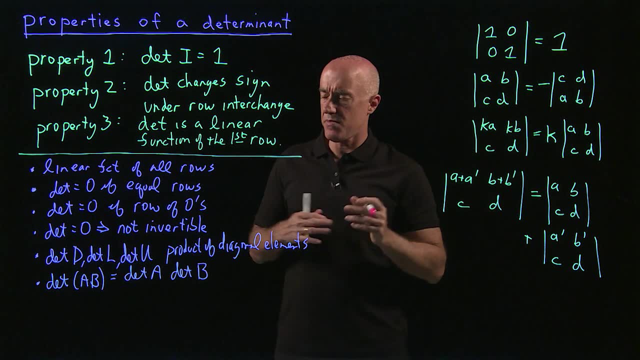 It's equal to the determinant of a times the determinant of b. So the determinant of the product separates into the determinant of a times the determinant of b. Of course a and b are n by n matrices. This is actually a somewhat tricky theorem to prove, but one can prove this based on. 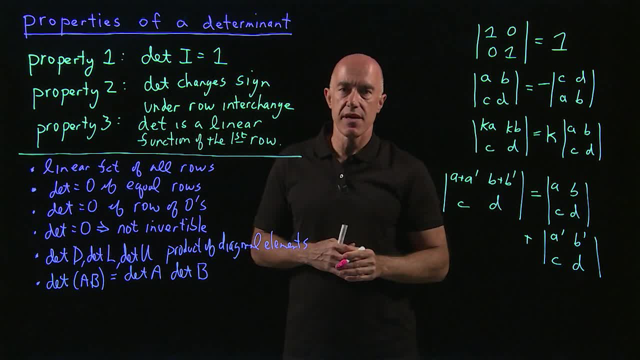 properties one, two and three and subsequent properties That one derives from one, two and three. Very useful. This is actually a very useful result And do not be confused: Determinant of a plus b is not equal to the determinant of a plus the determinant of b. 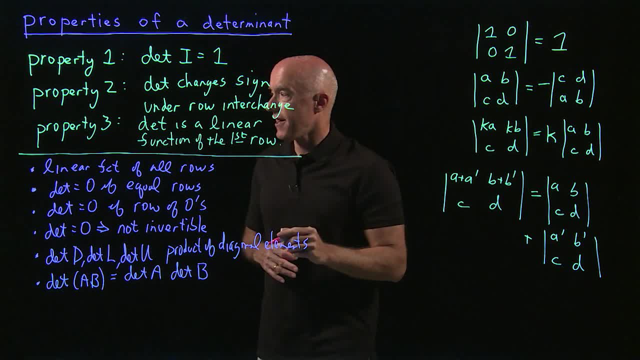 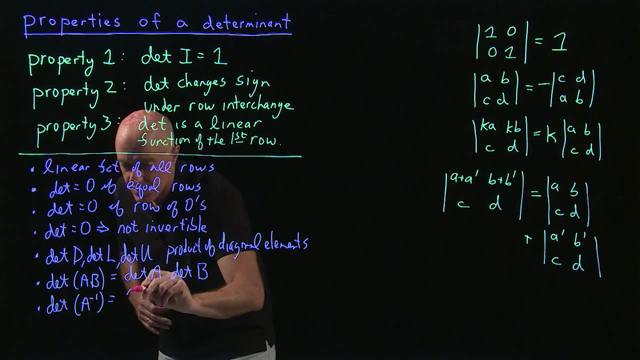 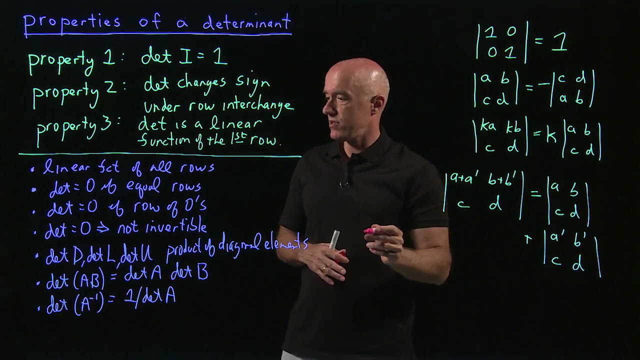 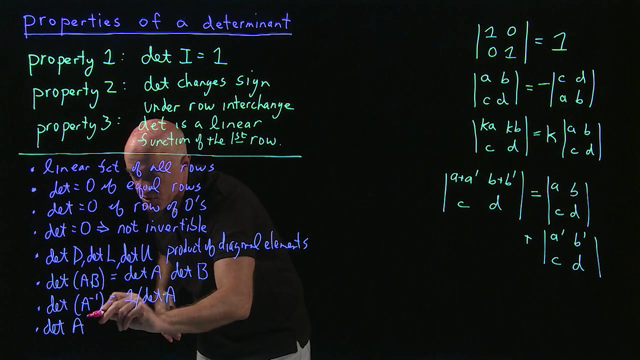 It only works for multiplication. The determinant of an inverse matrix, if a is invertible, is equal to one over the determinant of a. That's a nice result. And the last result that I want to tell you is that the determinant of the transposed 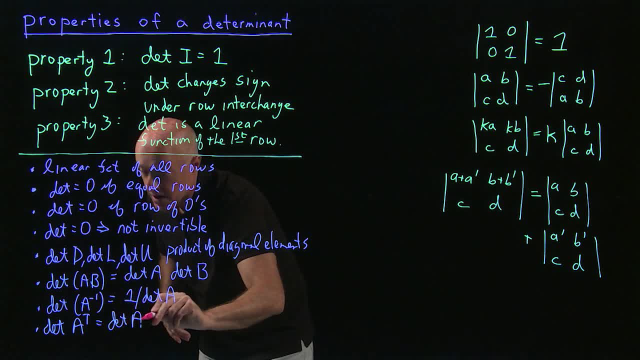 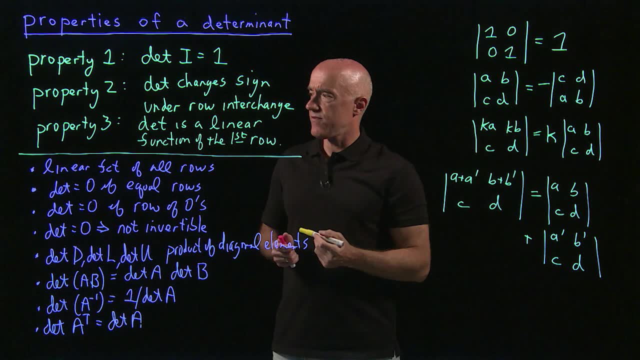 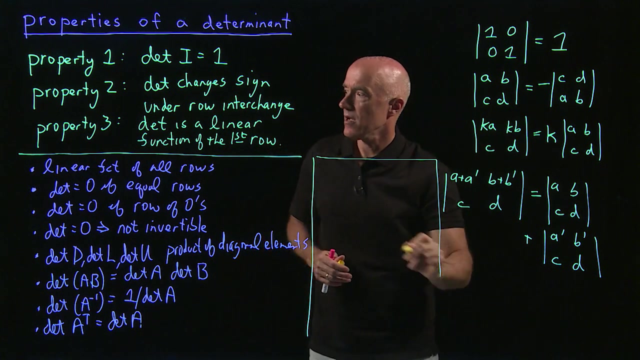 matrix is equal to the determinant of a. OK, So using all of these results that we have here and the properties one, two and three, there is a very nice and practical result, which is that the determinant doesn't change, Right. 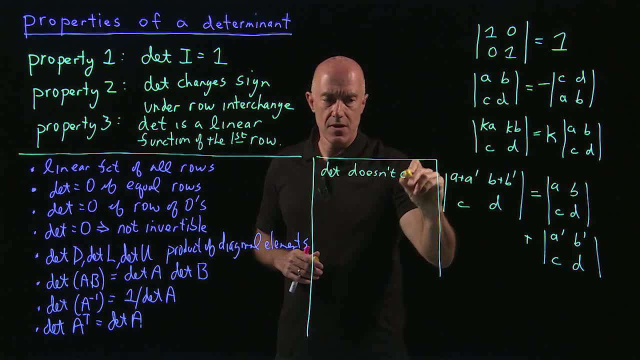 The determinant doesn't change. Determinant of a matrix doesn't change When you multiply a row by a constant. when you multiply a row by a number, a constant right A number, say, and add it to another row. OK, 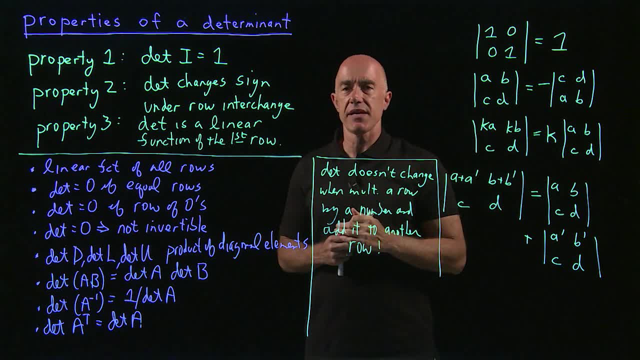 That's a very important property. So this is Gaussian elimination, right. You try to zero below the pivot by multiplying the pivot row by a number and then adding it to the row below the pivot In order to get zeros under the pivot. 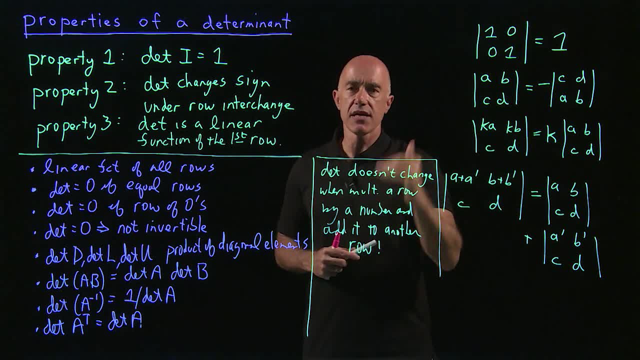 So that process of Gaussian elimination doesn't change the determinant of the matrix. So it gives you a method of computation where you can work on a matrix, reduce it to upper triangular form using this Gaussian elimination, and then the determinant is just the product of the diagonal elements. 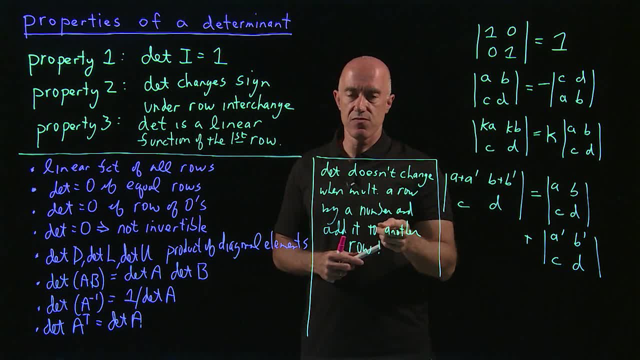 So, computationally, this is a very nice result. OK, This is a very important result. The difference with Gaussian elimination is that if you multiply a row by a number and replace that row, you have to take into account this property 3.. 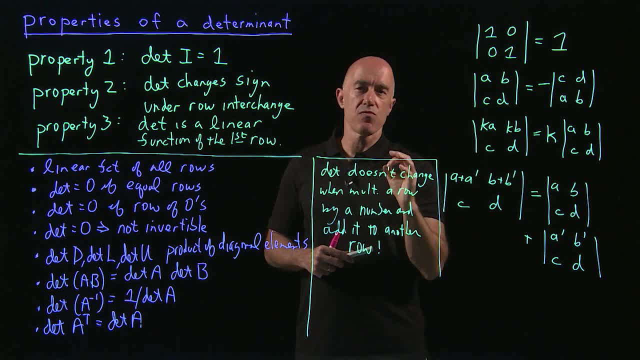 So that means that you cannot multiply a row by a number, that the determinant then will also be multiplied by the same number. So you have to be careful when you do that operation, OK, And also when you do Gaussian elimination. sometimes you switch rows. 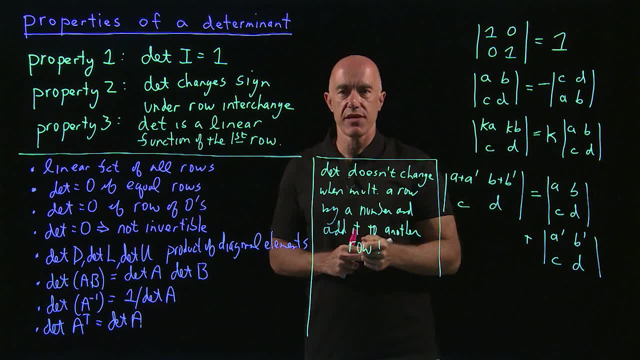 Here you can also switch rows, but then the sign of the determinant changes. So that's another operation. you have to be careful. But the standard workhorse of Gaussian elimination, where you multiply a row by a number and add it to another row, that doesn't change the sign of the determinant.